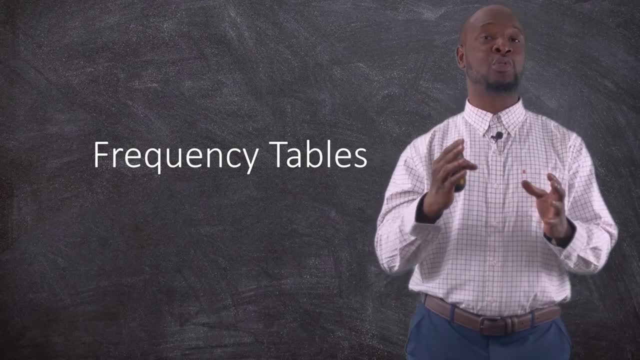 anywhere. I can only teach you what it is, because I know how to make it. You're going to see this classification on my own. You're not going to see this classification anywhere. I can, only can assure you, even if you see, it is not going to be in this format. so sit back and relax and 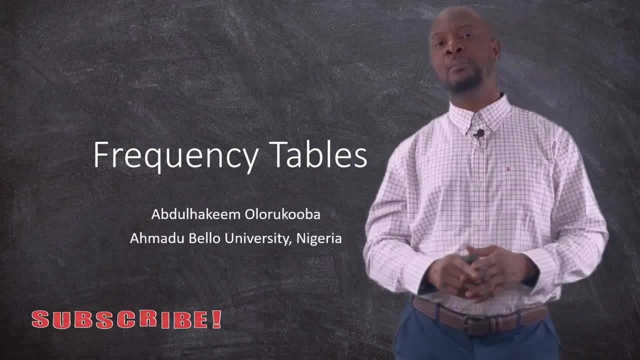 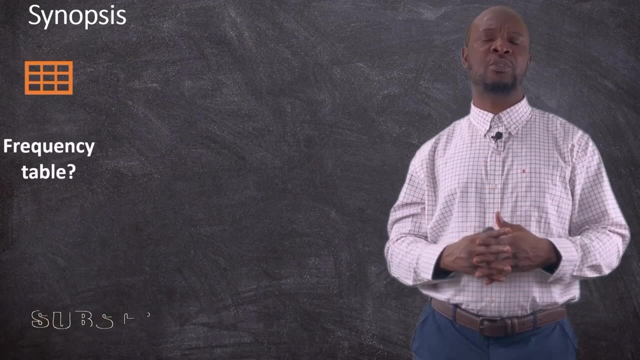 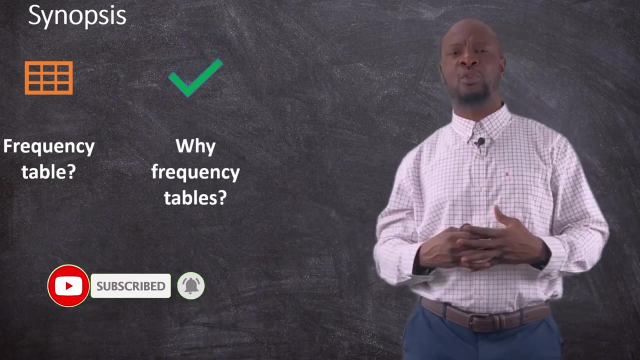 enjoy the ride. i'm going to use this very simple um outline to be able to take you from beginning, for you to understand some of these concepts. the first thing here is: what is a frequency table? all right, and then we're going to go into a description of why you need a frequency. 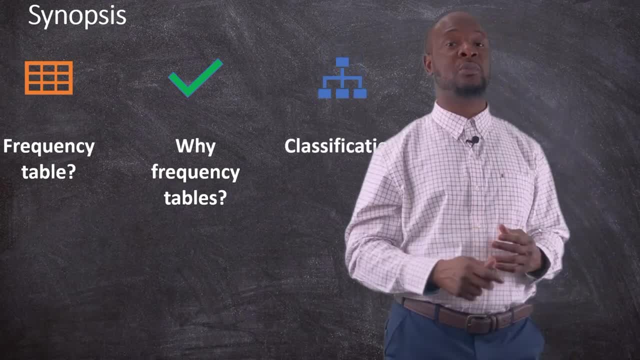 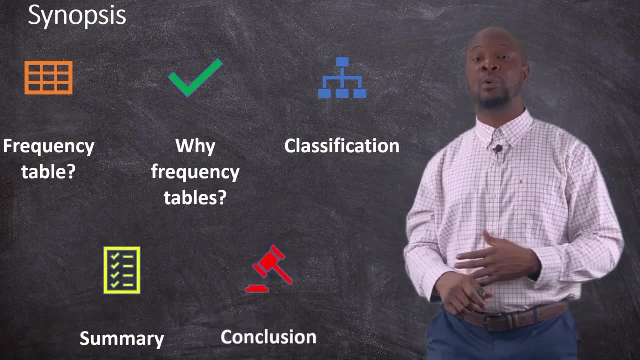 table very quickly before we now go into the classification. so stay tuned and stay till the end. i'm going to be talking about um, we're going to be summarizing what we have done and then, finally, we conclude. okay, shall we? what is the frequency distribution? before we go into this? 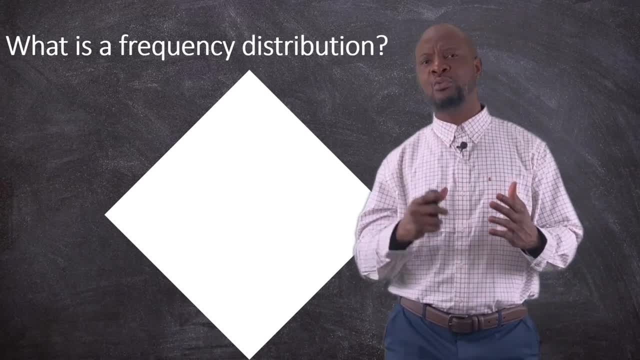 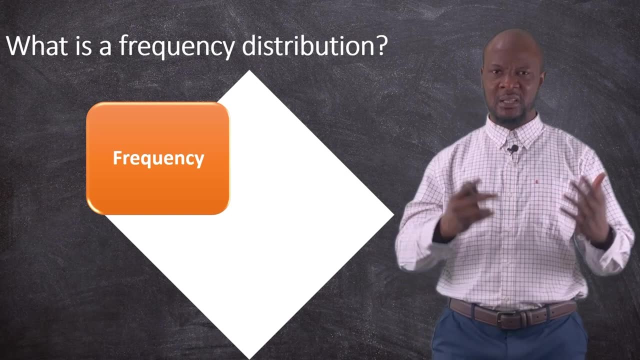 concept of frequency distribution. there are things that which you in which you need to know. the first thing is a frequency. when we say frequency, what do we mean? in layman terms, frequency is just the number of times in which something occurs. but remember, we're doing statistics, so in statistics, 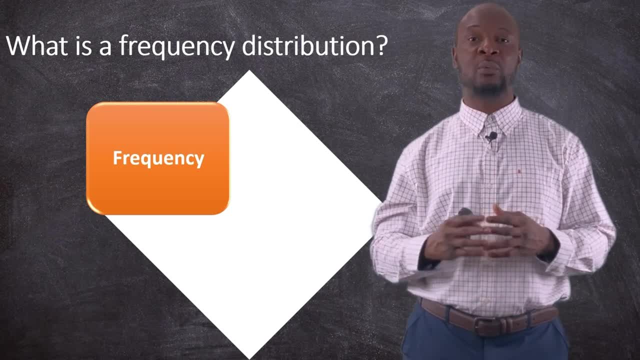 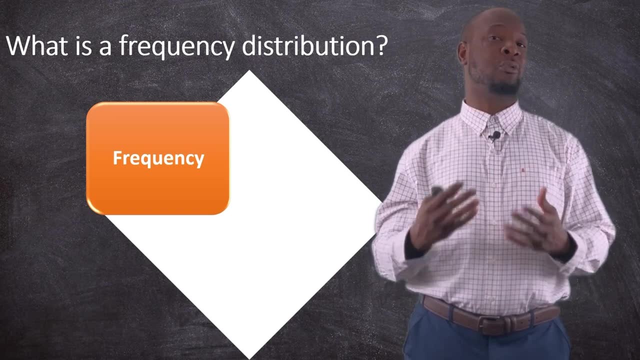 when you talk about frequency, it's usually in relation to a variable, and we remember that variables can either have categories or the variables can just have numbers or values. okay, so when we talk about frequency in statistics, we're talking about the number of times in which values of a particular 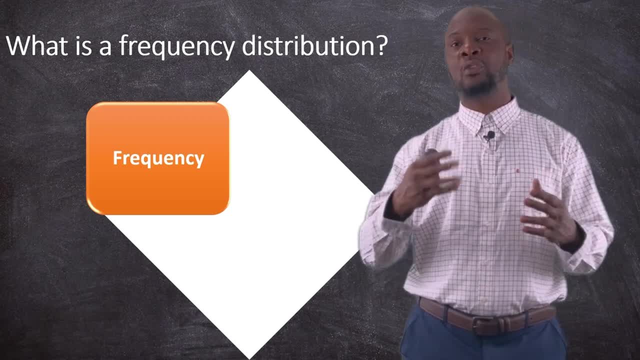 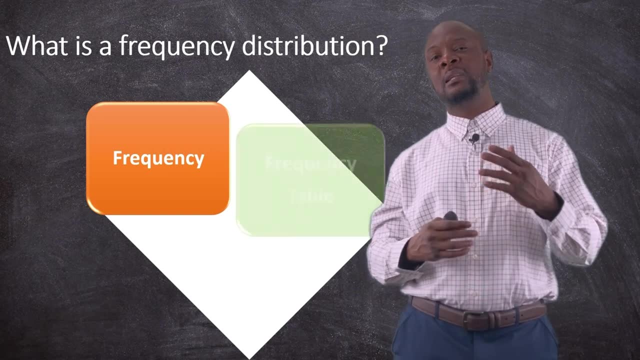 variable occur in the data set. so, if you have a data set, the number of times in which these values occur- the number of times in which these categories occur, is called the frequency- you'll be hearing frequency and it's going to be used with regards to a table, so you hear things like frequency table. 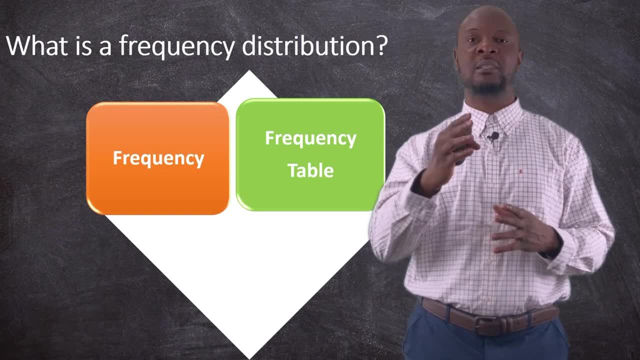 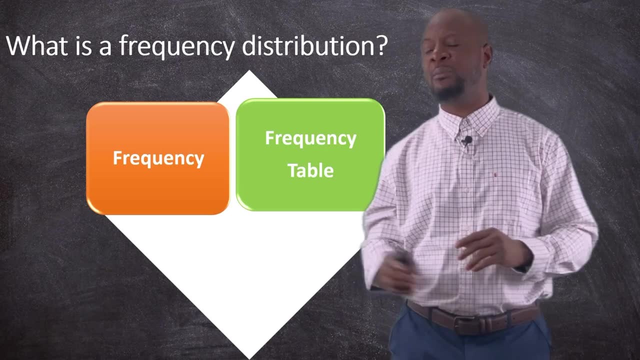 okay, a lot of people get confused when they hear frequency table. but a frequency table basically is a table that has frequencies, as simple as that, nothing too spectacular about that. okay, but when we come to the concept of distribution, that's when it starts to become a little funny. okay so, because when we talk about distribution in statistics, we're just 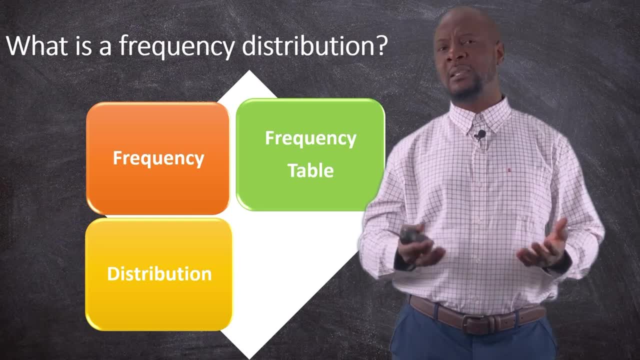 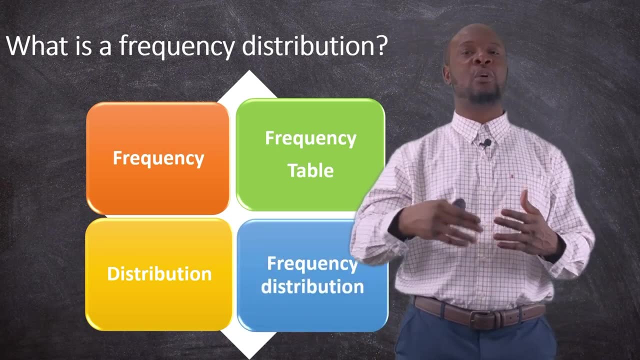 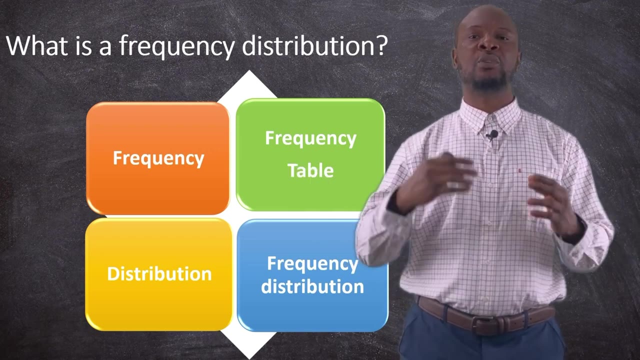 talking about a summary of particular characteristics, also of a variable this time. so that means when we say a frequency distribution, we're talking about the summary of the frequencies of a particular value of a variable. okay, in a in a given data set, all right. so a lot of people use these terms interchangeably. you can say: 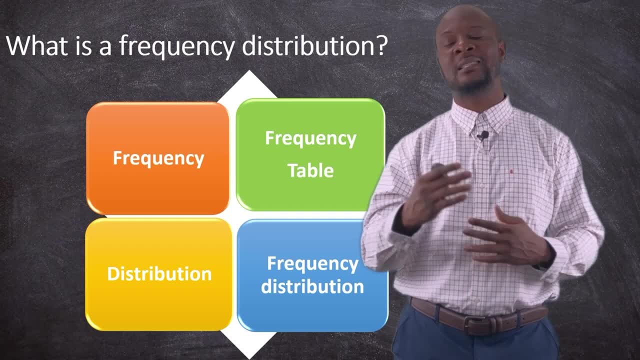 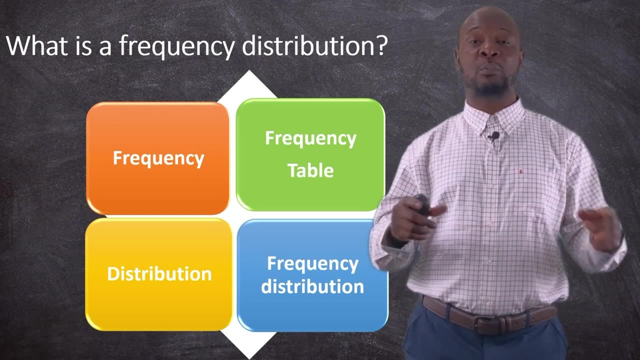 frequency distribution table. they can say a frequency table, or they can say a distribution table, whichever one you hear, i think they're just referring to the same thing. okay, so putting this out of the way, we're going to go straight to explain to you now. why do you need a frequency? 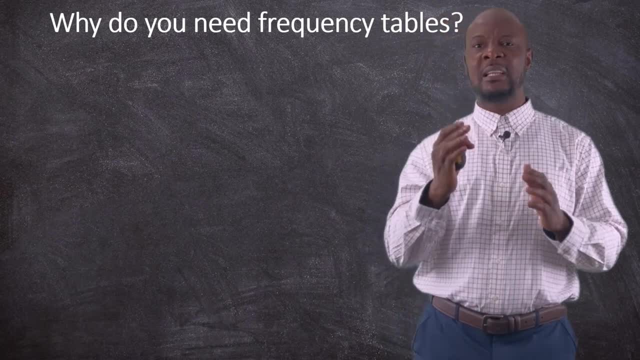 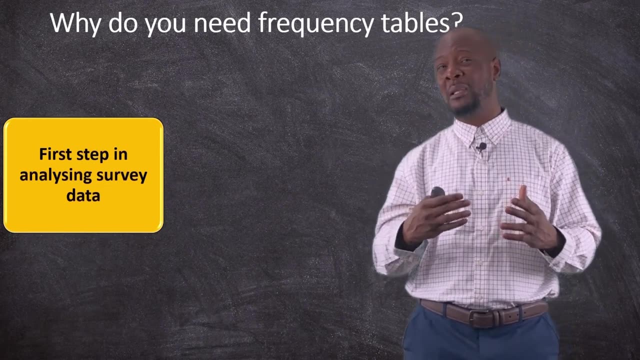 table. the frequency table is usually the first step in the kind of analysis and if you've done analysis before, you will hear your analysis, your analyst and you have you run the frequencies if you have any issues. once you run the frequencies you get a clear picture of what you're doing. so the first things that most of the times we do when we're 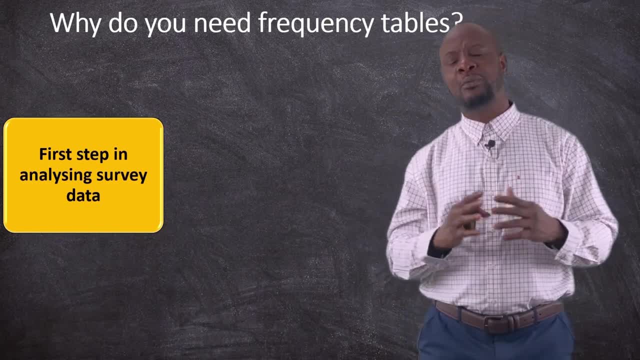 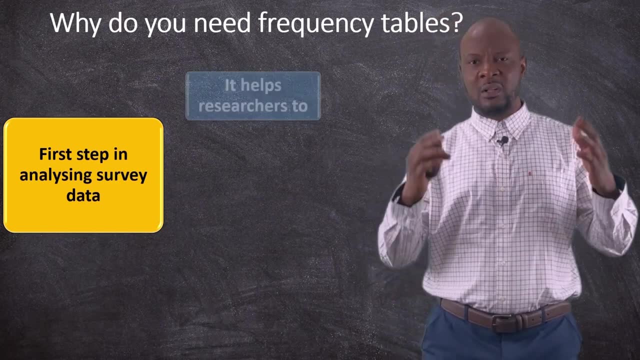 running analysis is to first do um the frequencies, run the frequencies and get a frequency uh table. what does this frequency table help researchers to do? number one: it helps you to organize. so you get organized because you can see everything in one small snapshot, because this table is like a 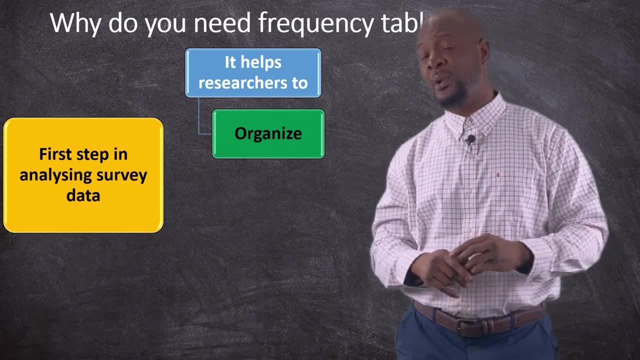 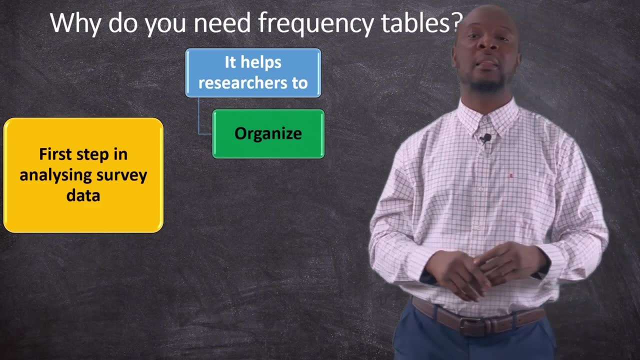 summary of all the frequencies, of all the different values in your particular um, of your particular table that you are trying to analyze. okay, it also helps you to summarize, like i've said before, and then, finally, it helps you to interpret the data in a way in which you can understand one of the other. 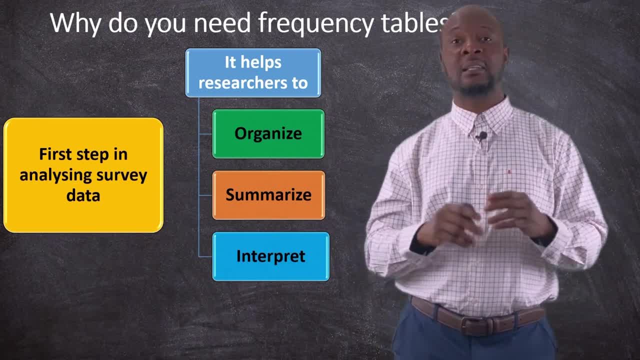 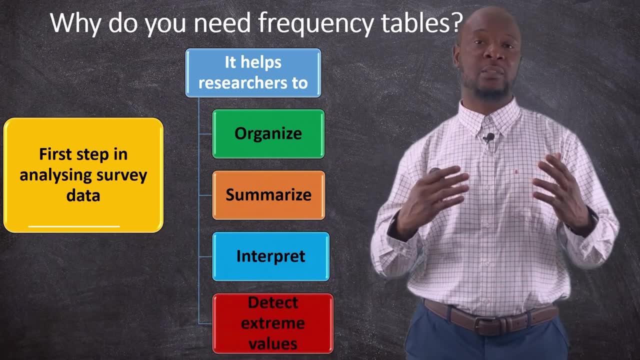 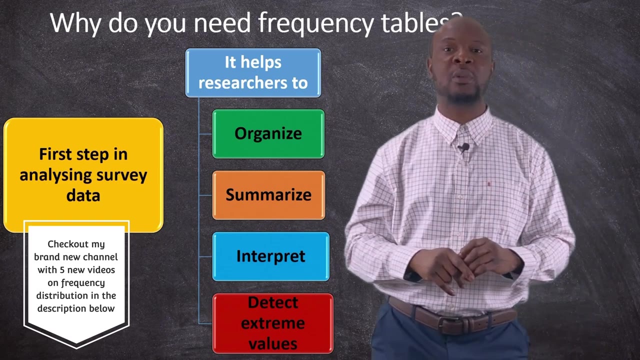 things. that is very, very nifty in a frequency table is that it gives you an idea of the variables that are actually um, it gives you an idea of the variables that are outliers, so extreme, uh, values. these are the uses of a frequency table. the next thing we're going to now go into proper. 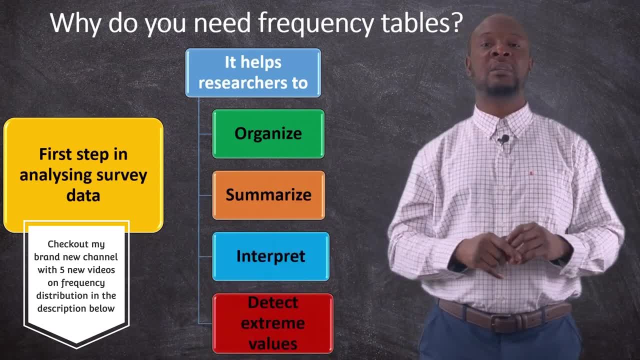 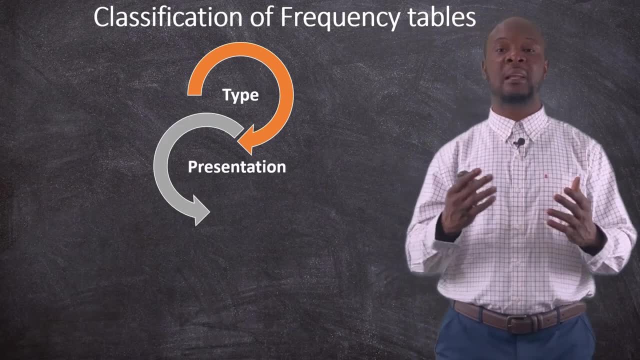 classification. so this is the classification i've been telling you about. you can either classify based on type, or you classify based on the presentation or the kind of transformation that you have, or, finally, based on the frequency, and you're going to see this as we go along into the 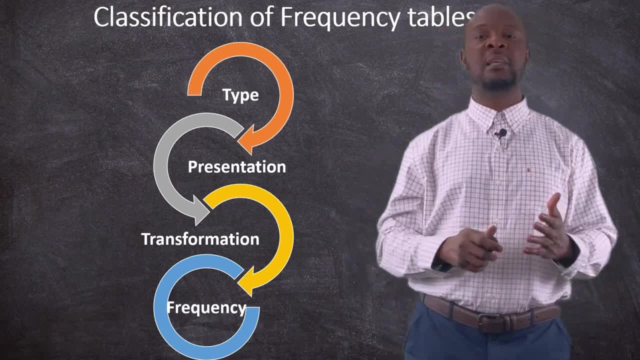 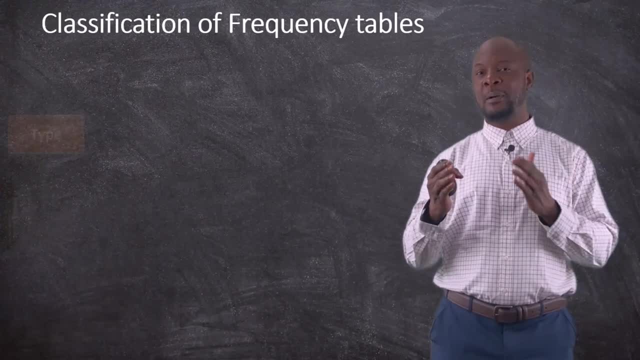 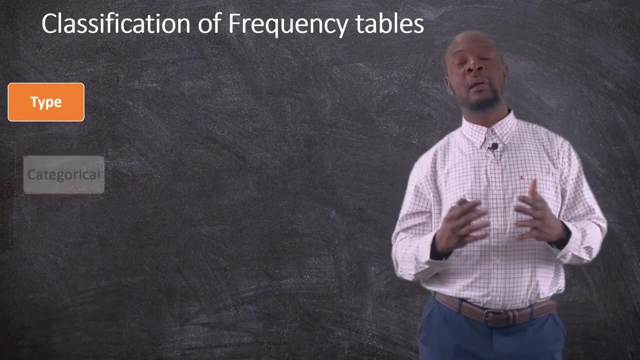 next slides. okay, so what do we mean by when we say classification based on type? so you can have classification based on type and this is based on the type of variable in which you are representing in the frequency table. so you can have something that is categorical or can have something that is um numeric. okay, so if the variable is a categorical variable, that 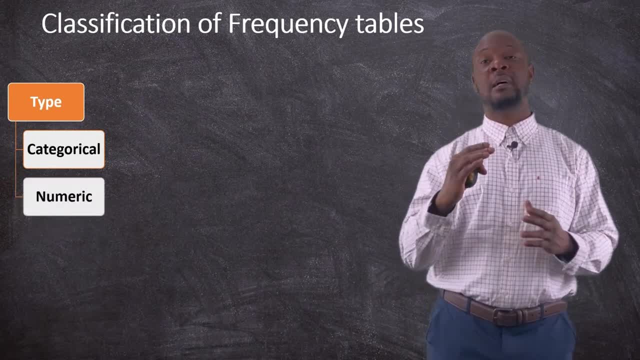 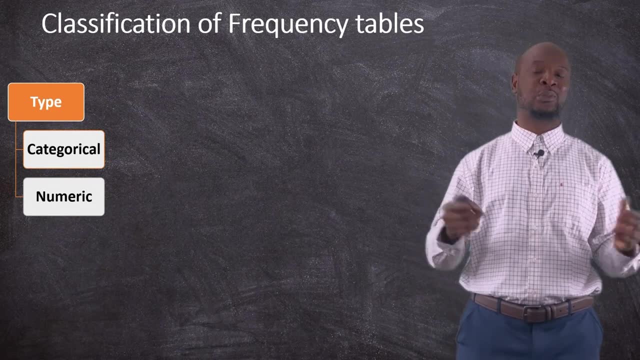 means he has categories or the variables. in numeric variable, that means he has numbers or values. then you can say a categorical frequency distribution or you can say a numeric frequency distribution. it's as easy as that. okay, the next thing is based on presentation, and when we talk about 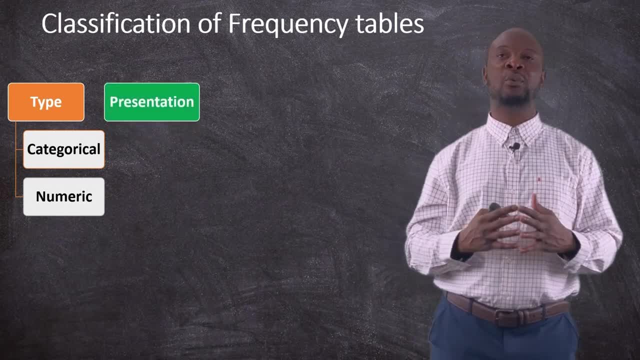 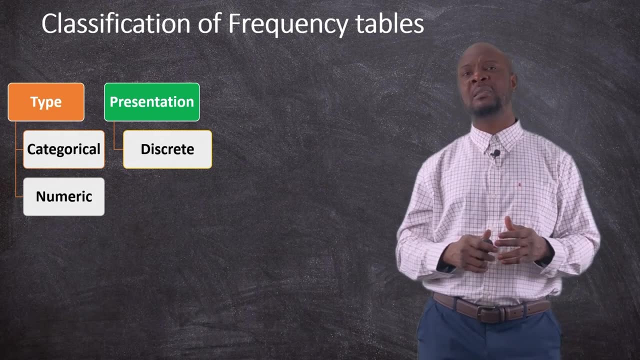 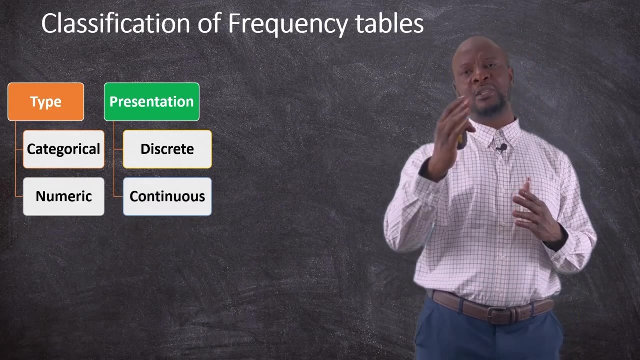 based on presentation is: either you have a numeric variable and this numeric variable is represented in a discrete format, so that means it has whole numbers- you have it in a format that is continuous, that means it has decimals, so you can have something that we understand as a numeric discrete frequency distribution. so it's not anything very difficult. 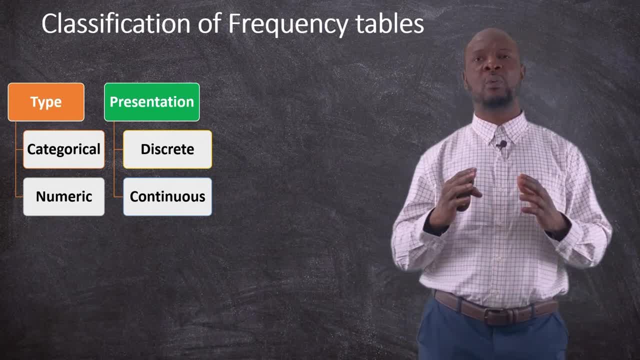 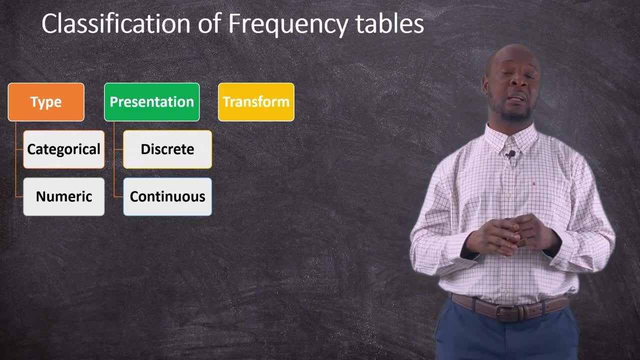 another way in which you can also classify this is based on whether you're going to do some form of transformation of of the frequencies, or your transformation of the values, or not. okay, so sometimes if you don't do any transformation, you have what we call ungrouped, and then, if you do, 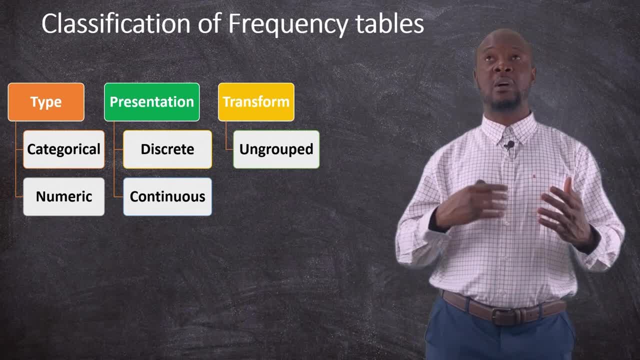 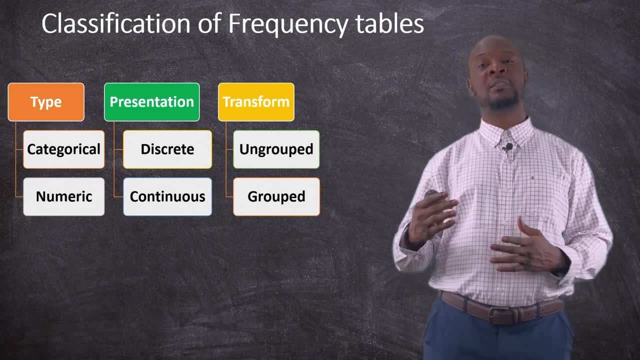 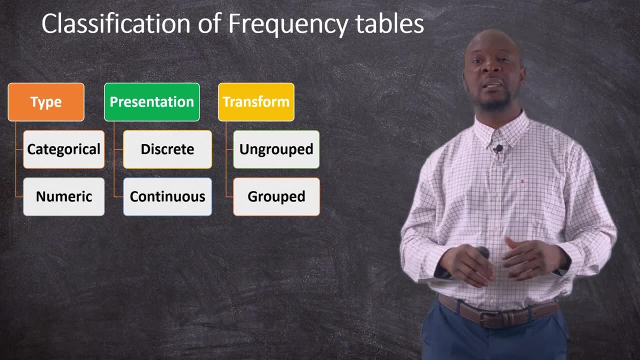 transformation. we have what is called the grouped. okay, so you have grouped. you can have a discrete grouped frequency distribution table or you can have a continuous ungrouped frequency distribution table. i am going to see all of this, you see, with vivid examples. the final one that we're going to be talking about is based on frequency, based on 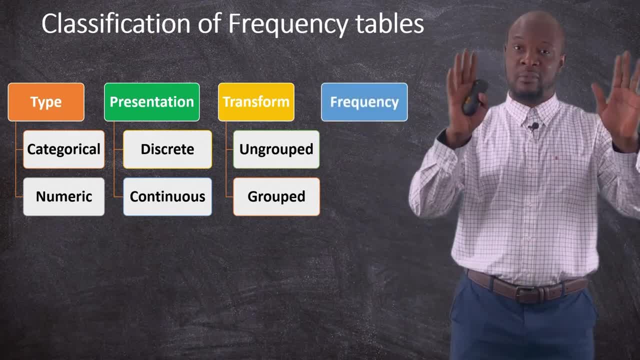 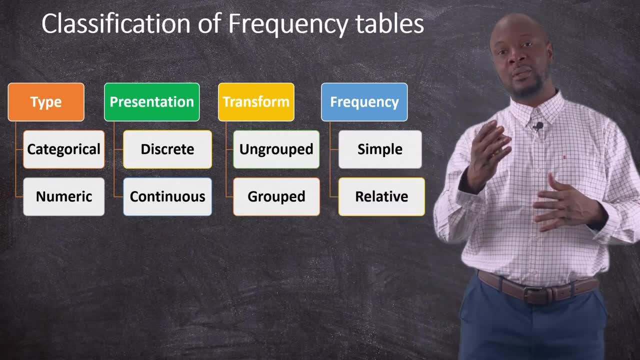 what you do to the frequency. so if you don't touch the frequency, you have a simple frequency distribution. all right, so what? if you touch the frequency, then you might probably want to do a kind of relative frequency on the table. so what that table is called a relative frequency. 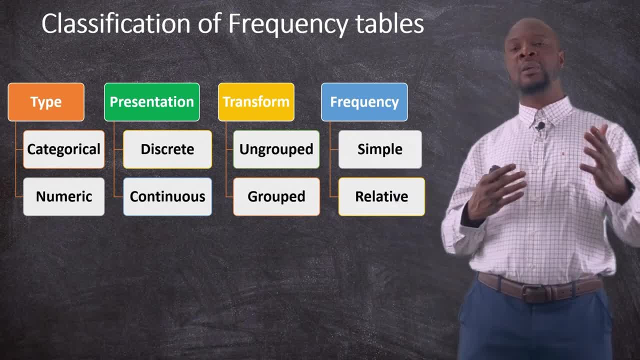 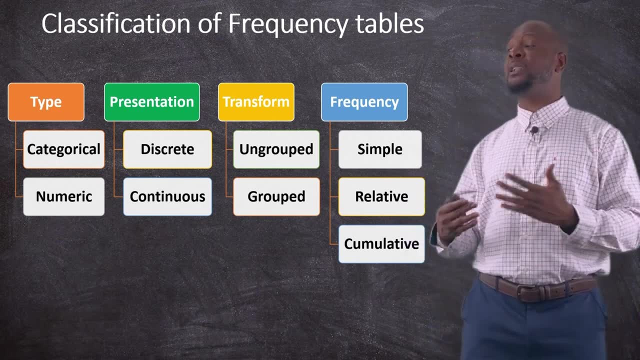 distribution table, all right. and then in another state you may want to do a cumulative frequency. so the table now is referred to as a cumulative frequency table. but you may go ahead to do some double barrel kind of arrangement where you do relative frequencies and the cumulative relative. 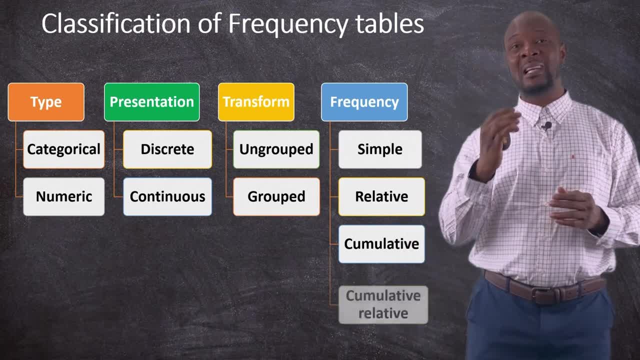 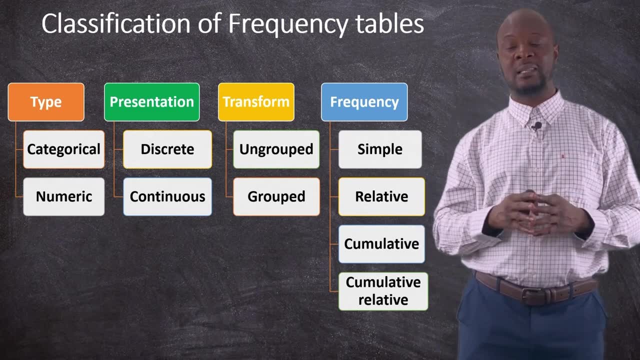 frequency and that kind of table is called a cumulative relative frequency table. so look at this classification. i assure you you're not going to see this anywhere, at least you're not going to see it the way it has been arranged like this. you may see it scattered in different textbooks, but i 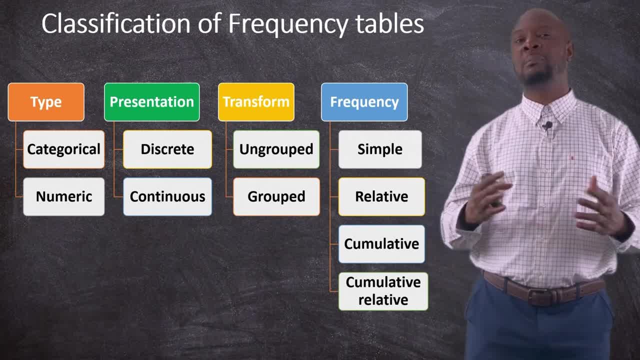 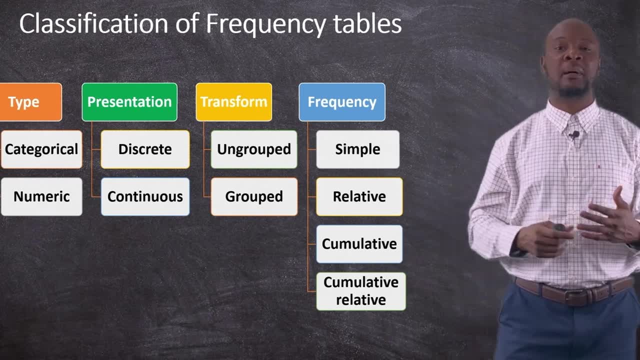 have been able to put it in a format that i've been able to use to explain to students over the past 10 years, and they understand. let's take this one by one. okay, the first thing that we'll be talking about is based on type, and you can have a categorical variable and, when you do, the frequency. 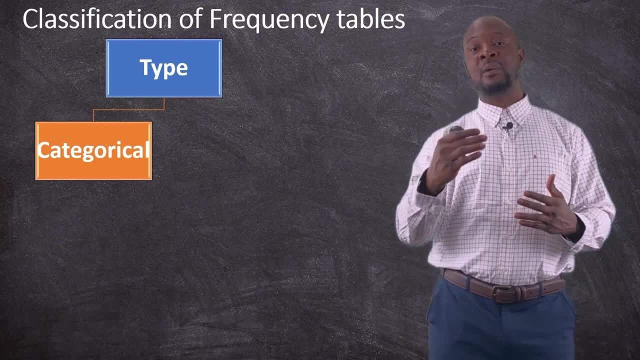 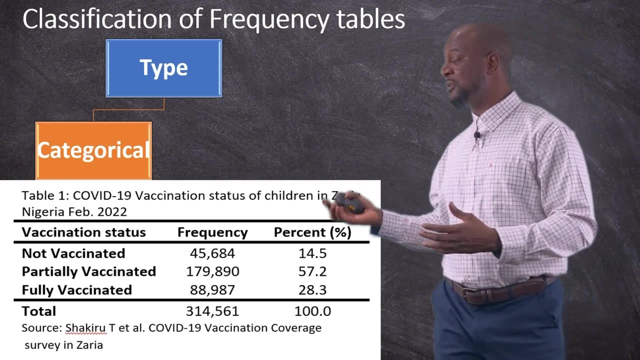 of that categorical variable, you have what is called a categorical frequency distribution. so the table is a categorical frequency distribution. look at this variable here. it's talking about vaccination status and we have three categories. so you have fully vaccinated, partially vaccinated and unvaccinated. okay, another. 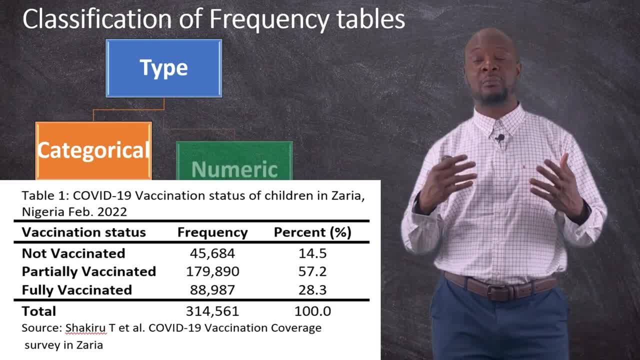 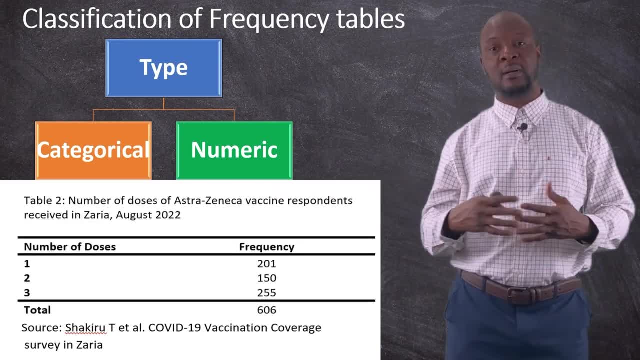 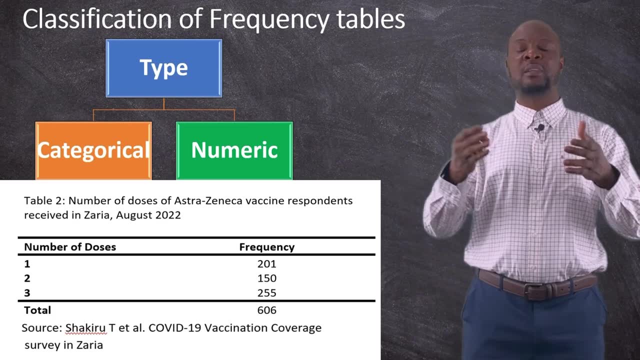 is the numeric or another type is the numeric. so when you have numeric data you can see that it's different. so this is data for number of doses of astrazeneca vaccinations and you can see some people had one, two, three and these are their frequencies. so this is a numeric frequency. 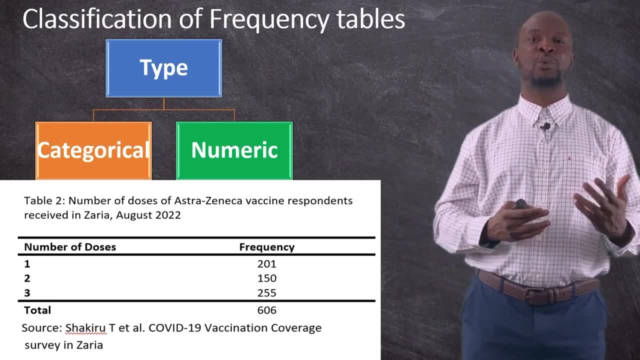 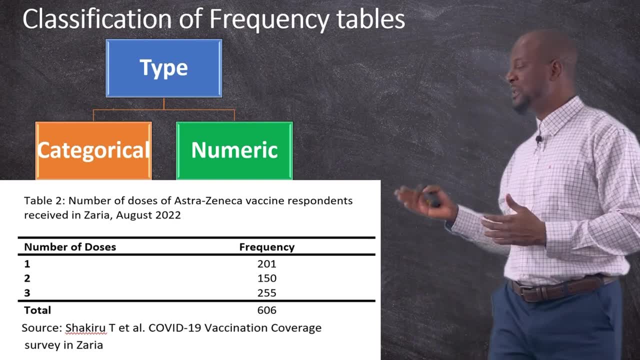 distribution. okay. so based on type, you can either have categorical or numeric, and you'll be seeing this a lot when you come to do your work. so we go to the next one, based on presentation. so are you as a discrete variable? so if the variable is a discrete variable, it comes with whole numbers. 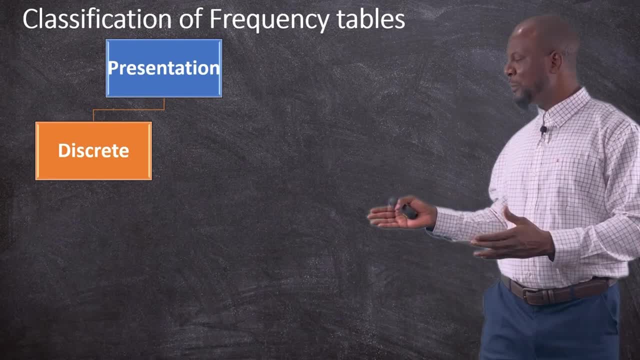 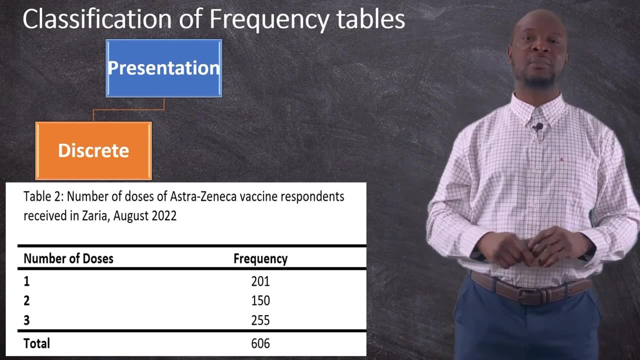 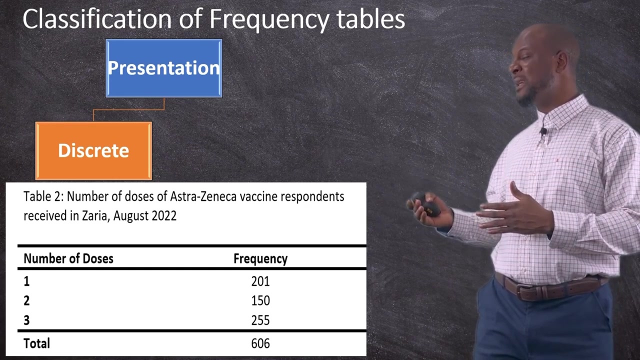 just like the previous example, you still have the same whole numbers and we can see their frequencies- one dose, two doses or three doses- and this is what we have. so this table is simply what we call a numeric frequency distribution, or a numeric frequency distribution that has is discrete. 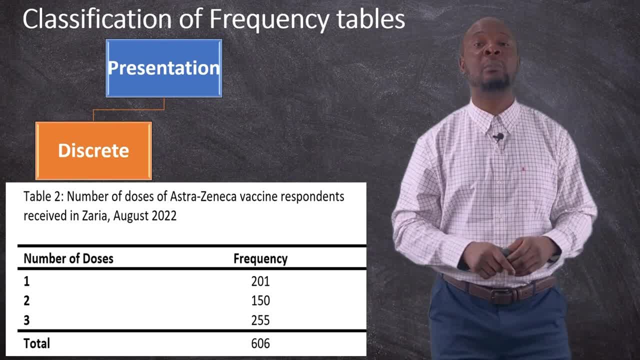 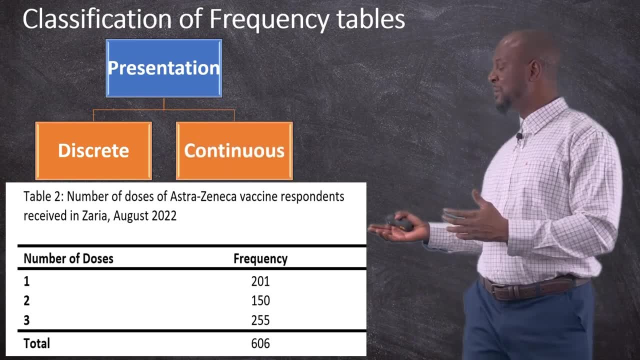 value. so we can call it a discrete frequency distribution. but still under the numeric class we have a number of different types of variables. so the next one we'll be talking about is continuous, and with the continuous the variable itself has decimal. so you can see the difference, so you can. 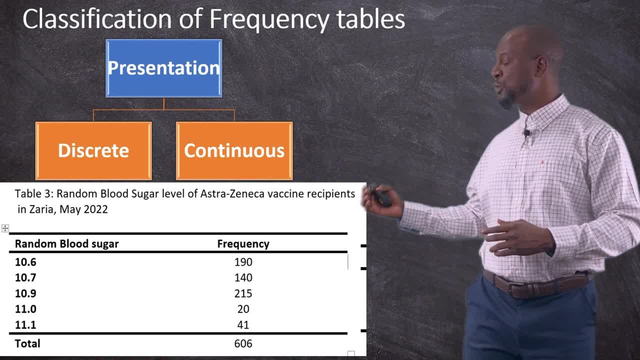 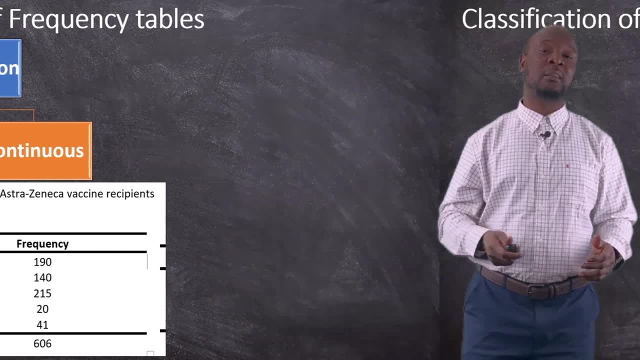 see the levels there, you can see the decimal uh points, and so this is called a continuous frequency distribution and you know it's of the numeric type. all right, no confusions at all. we go to the next one. the next one is based on the kind of transformation that you do. so if you do, 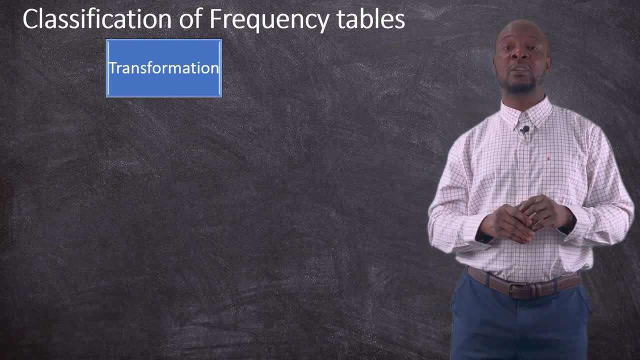 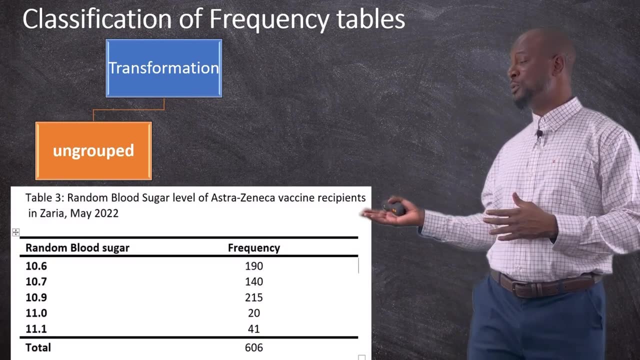 some form of transformation on the frequency or on the value of the variable, you can have something that is ungrouped if you don't touch it at all. so, like some of the examples in which we had before, we have a continuous distribution, but this is ungrouped because we didn't make any 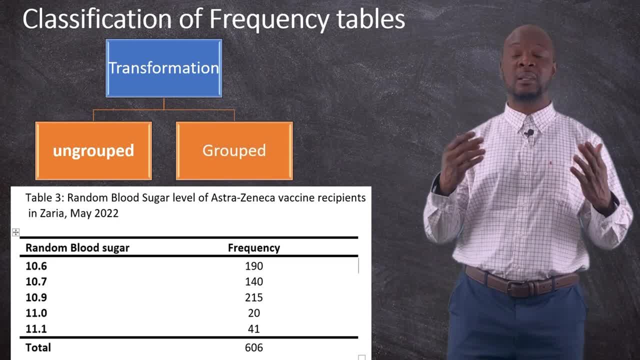 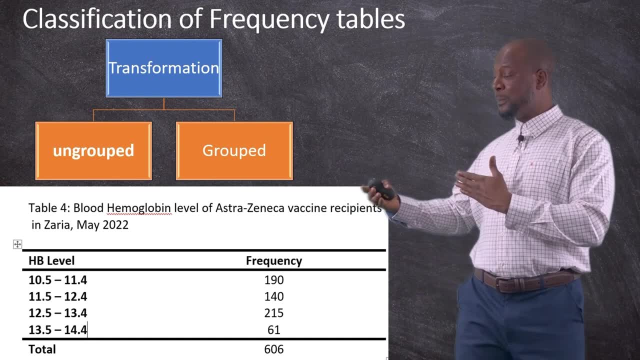 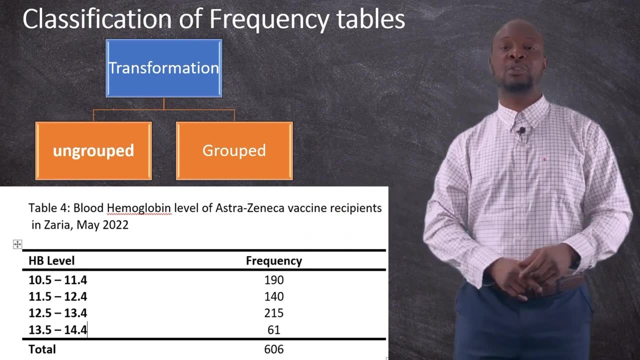 grouping. you can have another situation like this, which is the grouped one and the grouped one. you can see that we have been able to group the values into some particular grouping. so this is a continuous one, but it's grouped. so this is a grouped. frequency distribution table of the 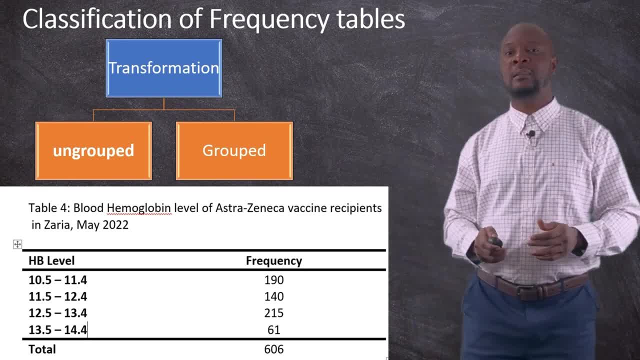 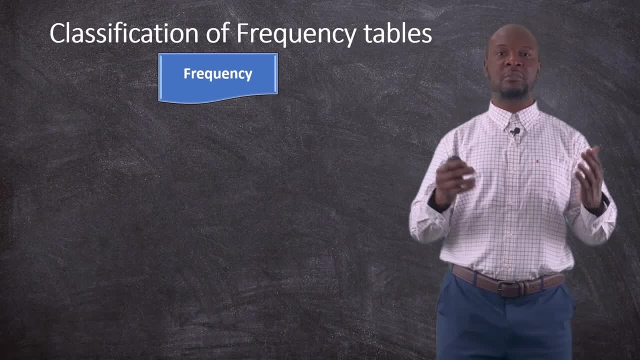 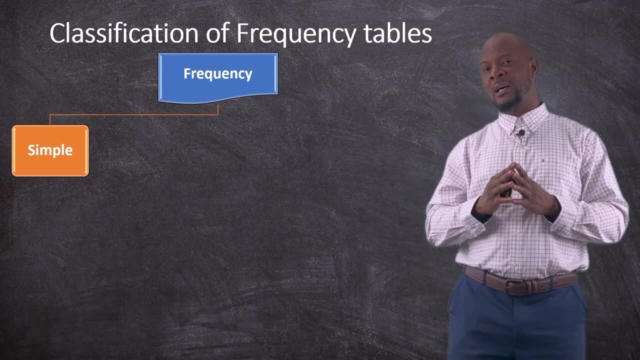 continuous category, so i hope this helps is getting clearer and no confusions up to this point. the last one is based on the frequency and so if you, if the frequency is, you can have a situation where your frequencies are just exactly the way you are presenting the frequencies as you have seen them. you are not. 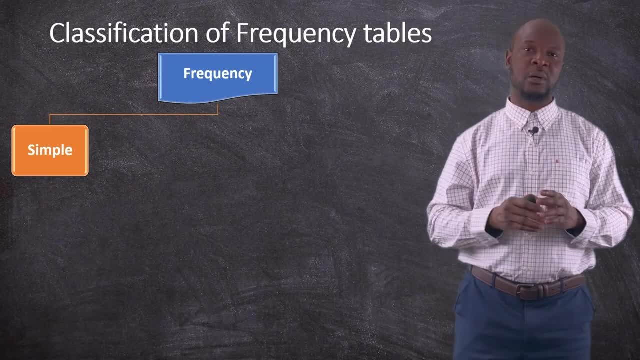 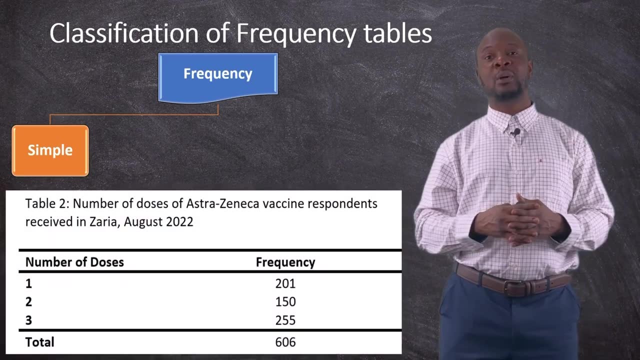 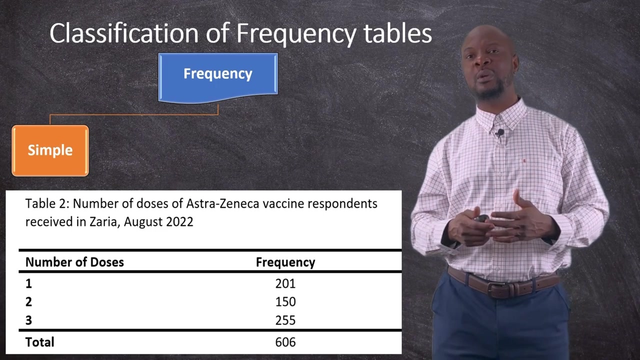 making any alterations to the frequencies themselves. so, and when you are doing that, what you have is called a simple frequency table. an example is this table that we have. so you have a simple frequency table here, where the frequencies are presented exactly as the way as as we we find it, but if we make some form of transformation to the frequency, we can have. 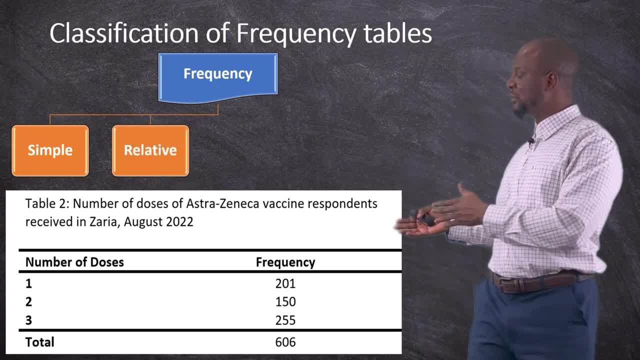 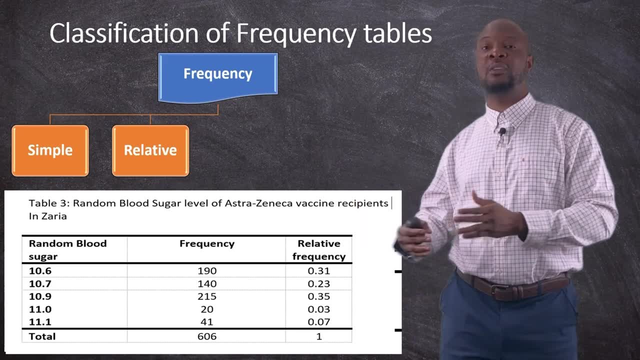 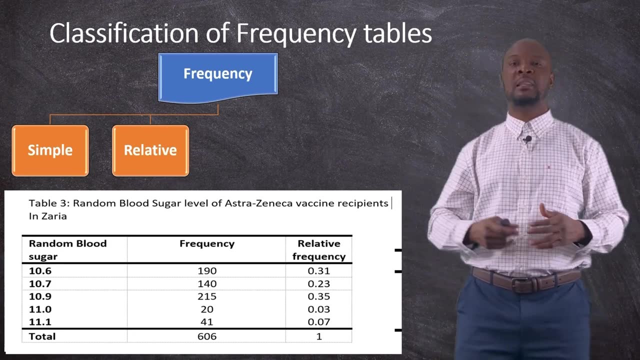 something that is called a relative frequency table. so you have a table that has frequencies and has relative frequencies, which is just proportions, you know, it's the same relative frequencies that people convert to percentages. and then you have a table that has uh, frequency and percent, okay, and then you can have cumulative frequency, and this is a situation where you put 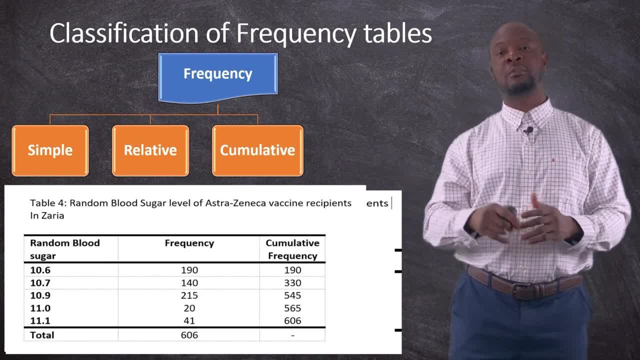 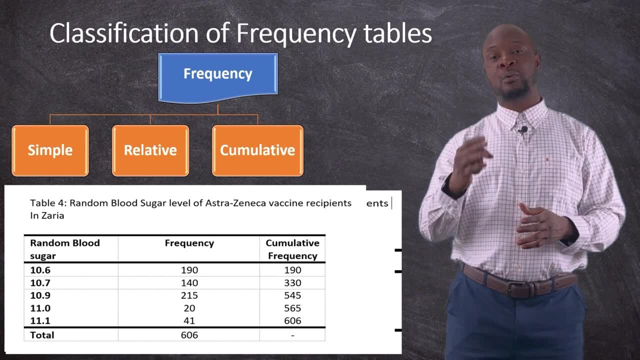 the cumulative effect of each of the frequencies. okay, and so you have a cumulative relative, you have cumulative frequency table. so this table, this example of this table, is a cumulative frequency table. well, you know, you can go ahead to do what is called a cumulative relative frequency and the cumulative relative 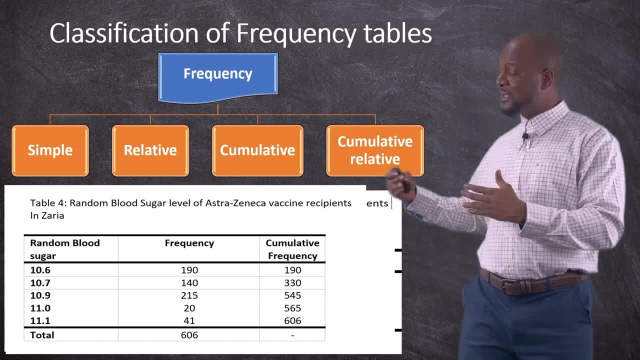 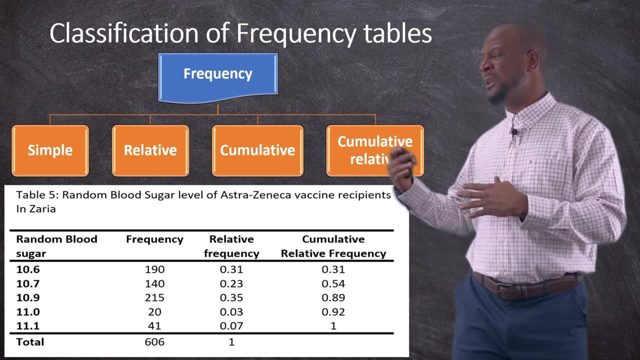 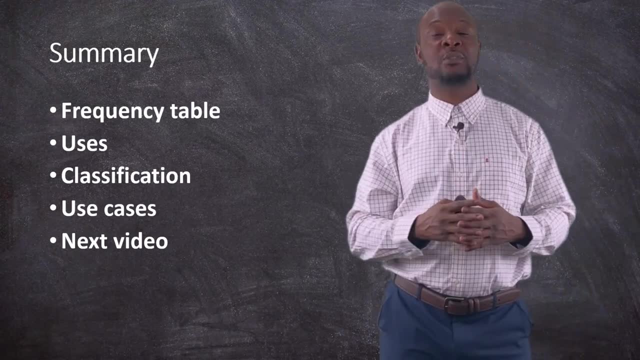 frequency- here the cumulative, the relative frequency. we now work on the uh and show the cumulative effect of the relative frequency. so here you have a cumulative relative frequency. okay, in a nutshell, we have been able to talk about the different categories of these classifications. we talked about what a frequency table is. i told you more about it in the previous videos and 2020. if you would like to see similar classes. we drastically increase the channel analysis, the wah, to some of the topics in the previous material video. but be sure you take me a quick word of advice, so i'll leave some��록 for this video, for those who like channel analysis and those who estoy am觤h off. 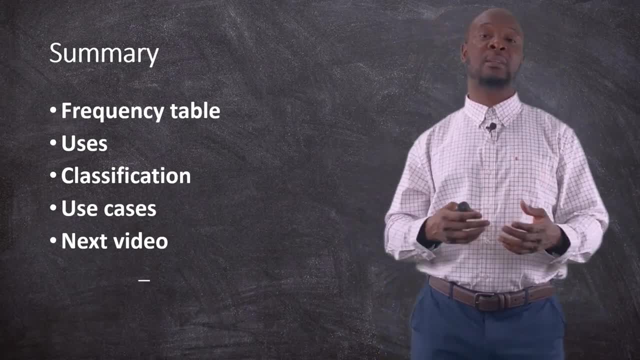 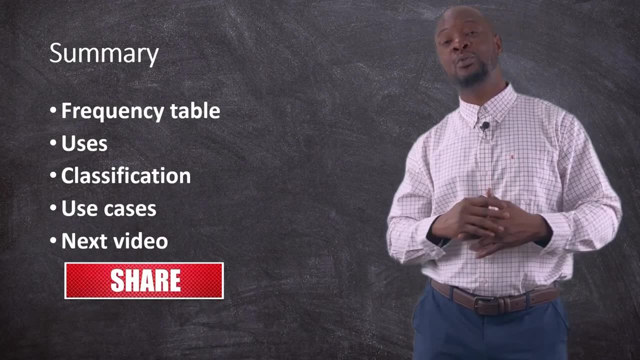 that's my way of going, while just watching industry and woodwork. i hope you also gain some understanding about the. I told you the uses of frequency table, where you can use it to organize, summarize or even look for outliers in your data. And then we have also been able to talk about all the different classifications and I gave examples of use cases. 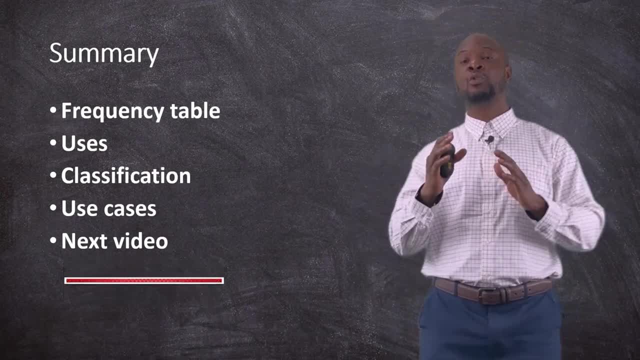 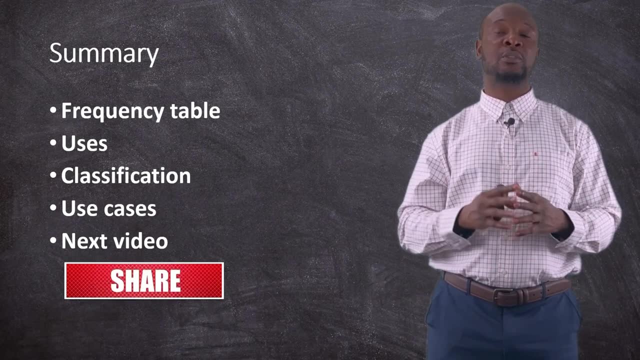 In our next video, I'm going to show you how to construct a grouped frequency distribution table. So if you gained value in this video, please don't forget to hit the like button, And then, if you have not yet subscribed, this is your time to subscribe. 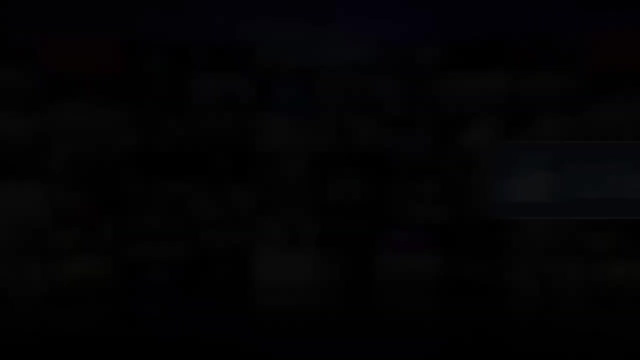 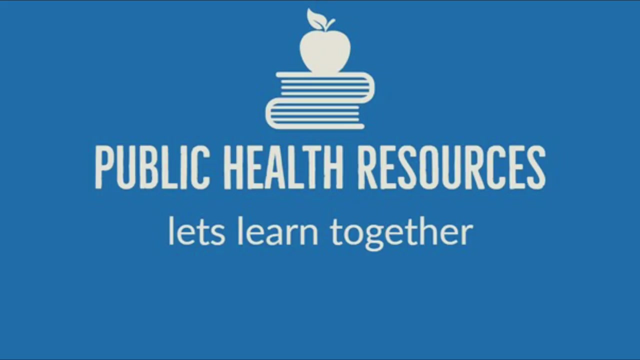 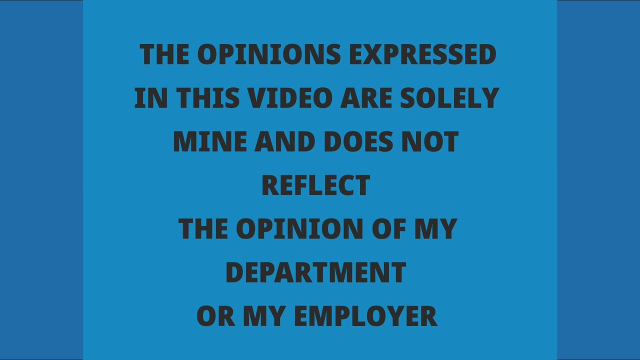 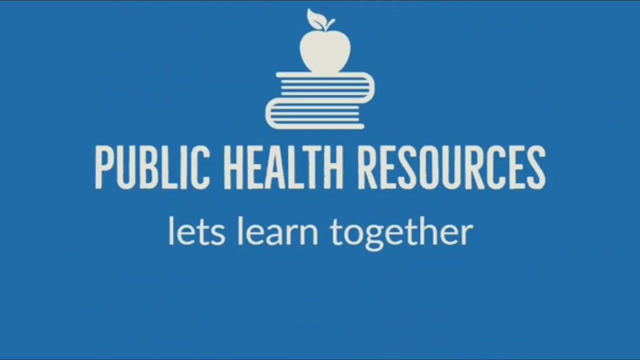 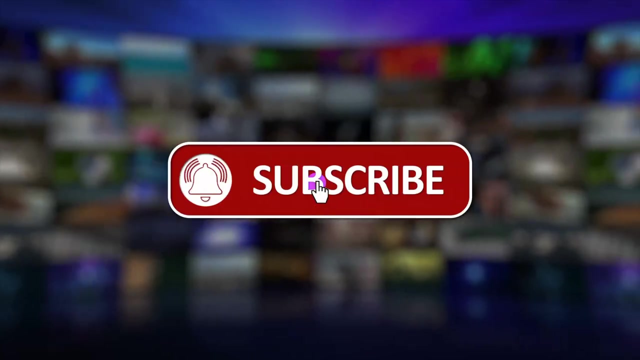 See you in the next video. Until then, peace. Thank you for watching.